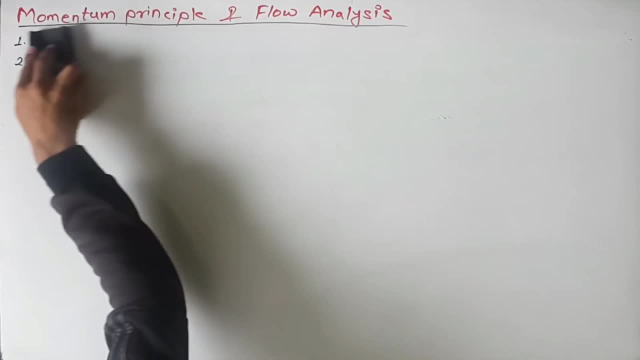 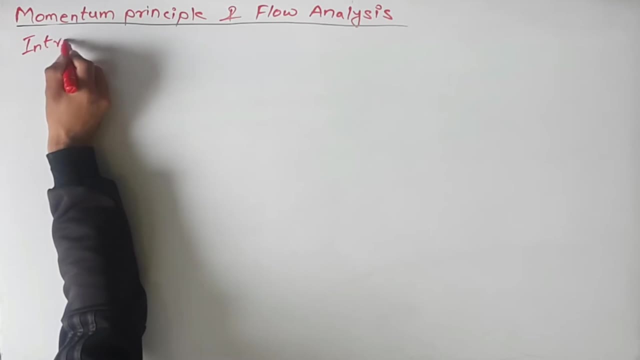 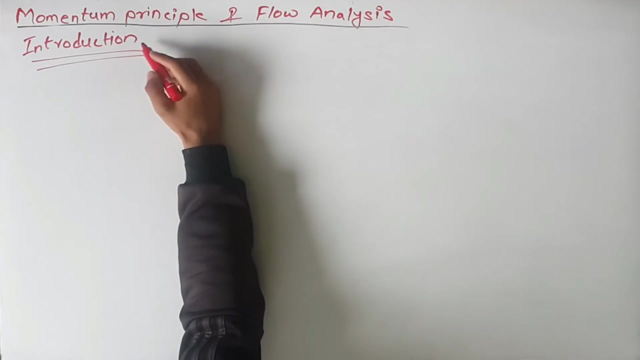 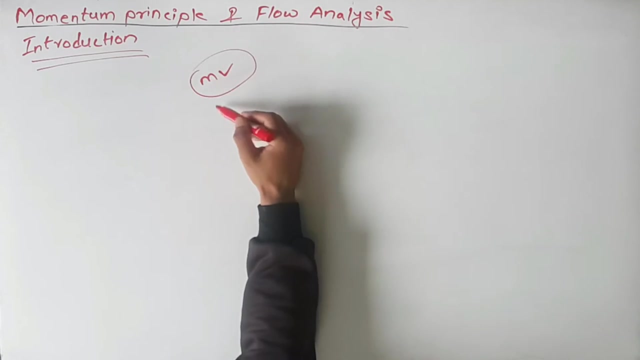 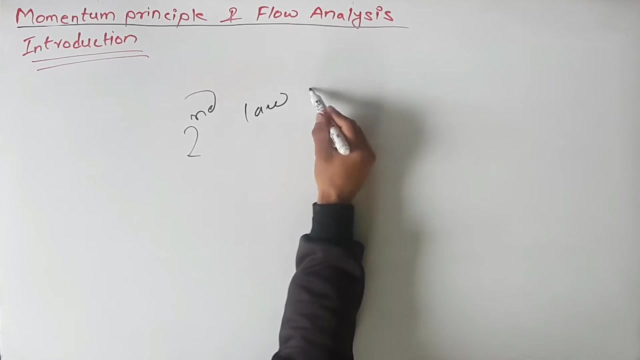 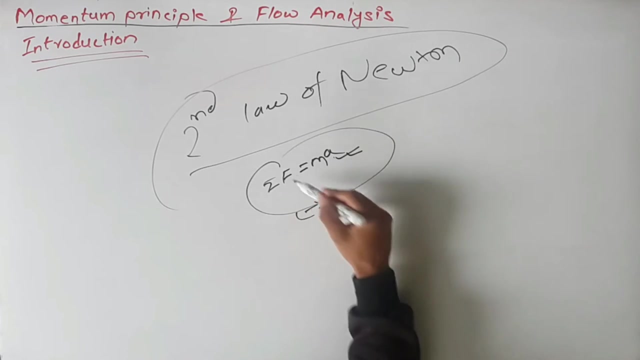 Here we have to study what is momentum first. Momentum is the product of mass and velocity. But in fluid mechanics, what mass is used in the flow analysis? So, in case of solid mechanics, we use this. And in case of fluid mechanics, we use this mv in different way. So, momentum equation is the statement of Newton's second law. We have studied second law of Newton. What this second law tells? Newton's second law relates the sum of forces is with acceleration. And this acceleration takes place in the direction of the force. We use this Newton's second law for flow analysis. Here is mass m. We use the mass mv which is moving in the solid mechanics. But in fluid mechanics, what mass is moving? 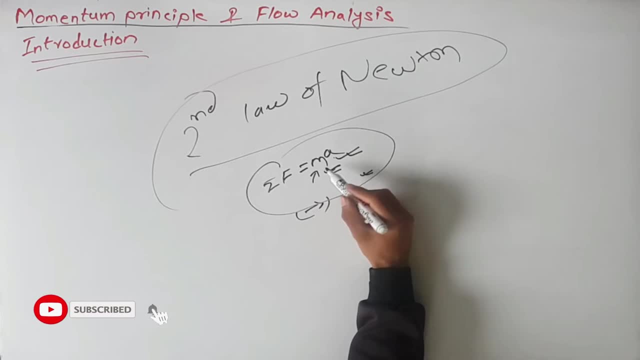 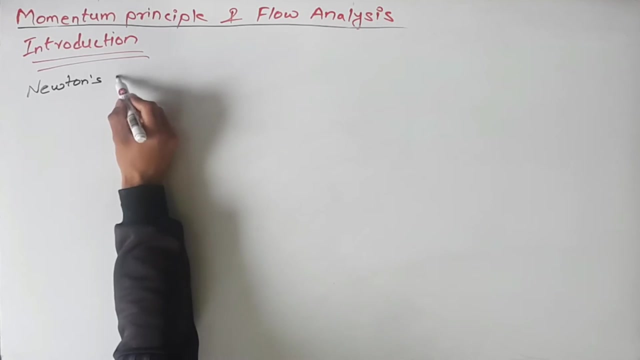 So, we use this equation for Newton's second law in different way. So, let us write what is Newton's second law? The statement of Newton's second law. This is the moment constant. This is the moment constant. And this is the moment constant. So, this is one moment constant. 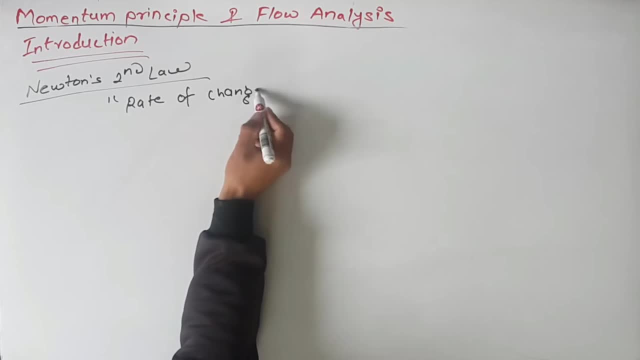 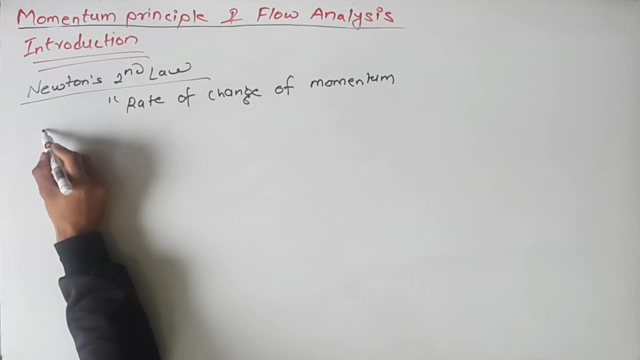 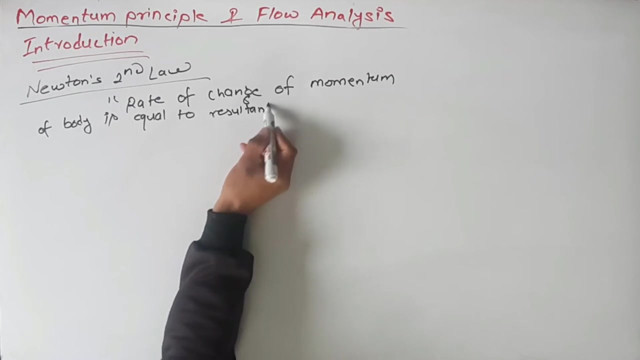 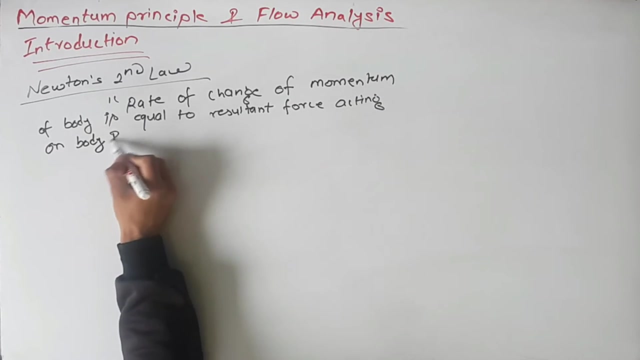 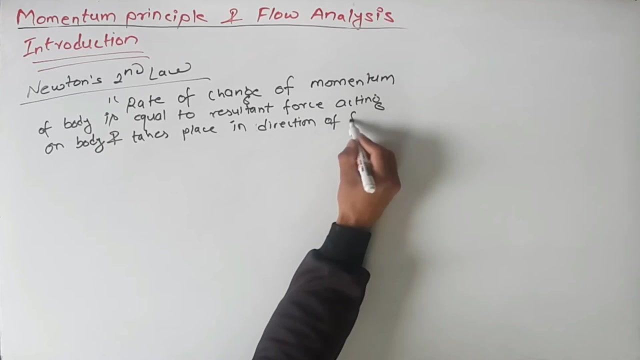 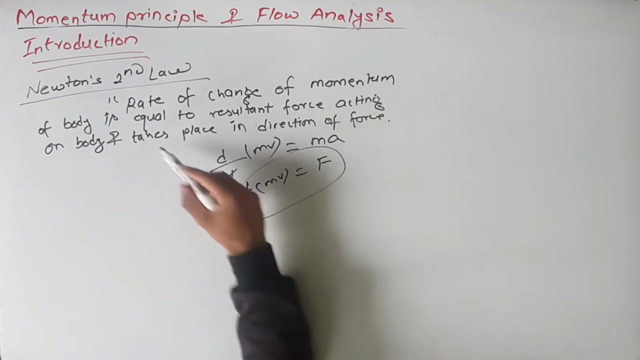 rate of change of momentum rate of change of momentum of a body is equal to resultant force acting on the body takes place in the direction of force and this is d by dt mb rate of change of momentum ma net force this is equal to d by dt mb equal to f this equation is this 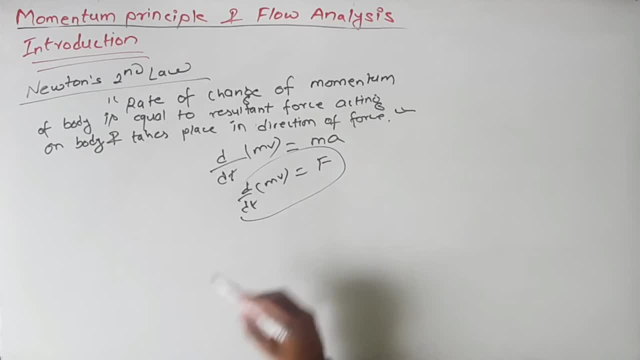 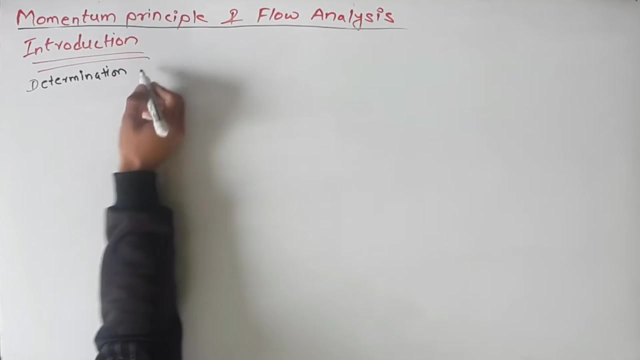 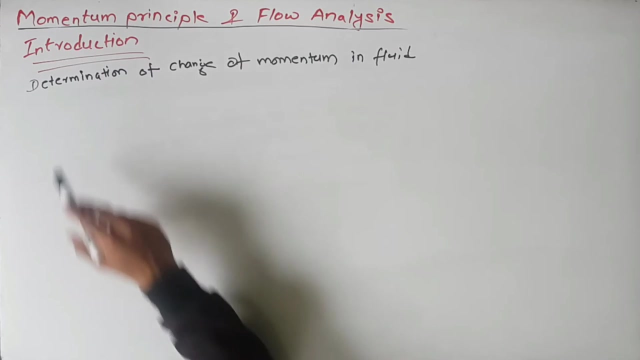 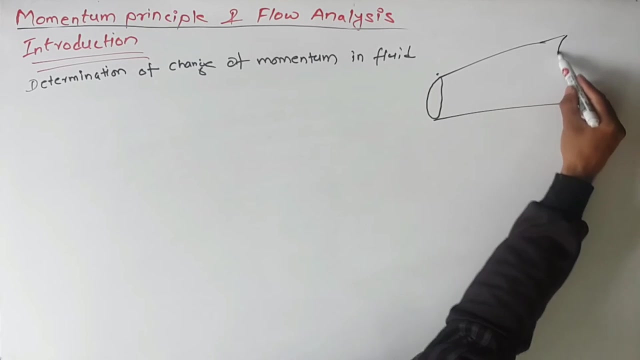 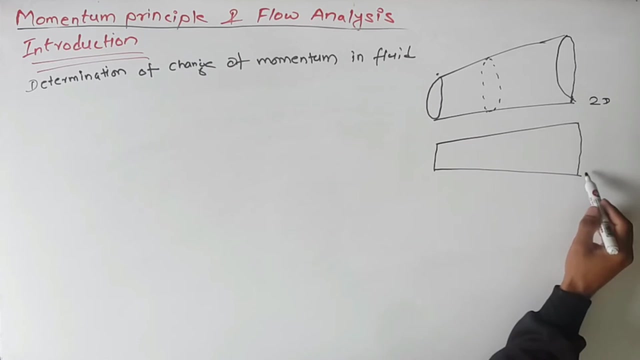 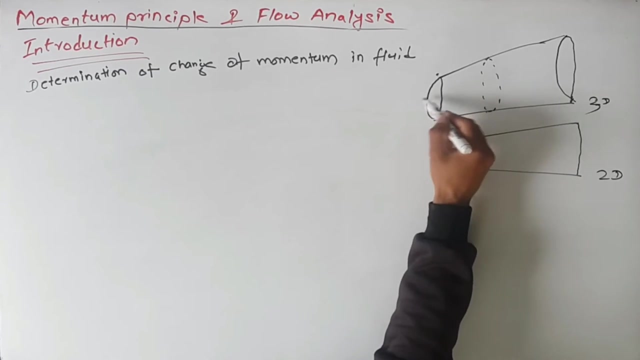 we have to verify this in case of fluid how this is possible in case of fluid determination of change of momentum in fluid first of all we consider a stream tube i will make a stream tube in 2d we can also make this is the 3d view here 3d view and this is 2d view your area of cross-section let me show you the area of cross-section 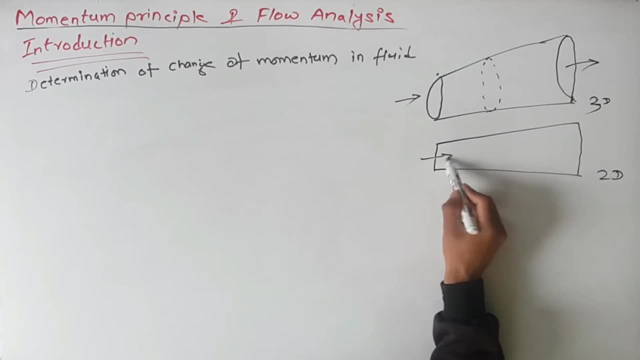 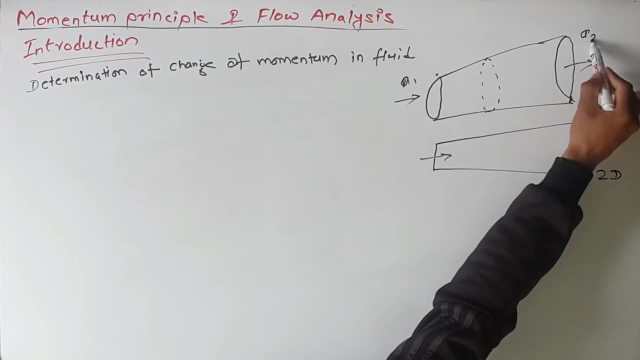 so here this is inlet and this is outlet 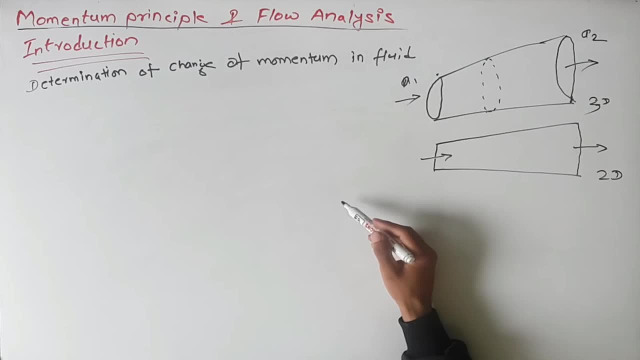 here area is a1 here a2 area is increased and velocity of flowing fluid is b1 here here v2 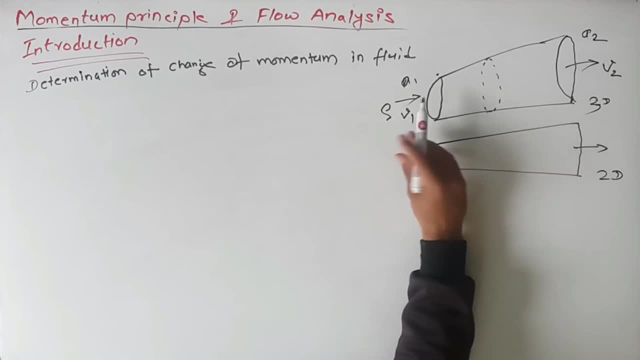 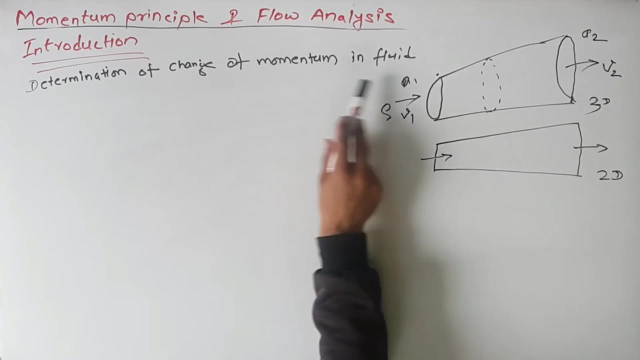 let the fluid or liquid of density rho flow across the fluid stream tube we start our determination of change of momentum in fluid by assuming this 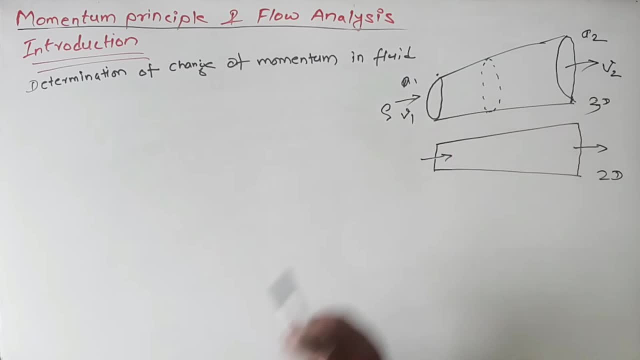 steady non-uniform and continuous flow what is the steady flow or we have to understand steady flow steady non-uniform flow means condition change from point to point but the parameter such as velocity area cross section pressure these are change but do not change with respect to time while flowing this fluid of density row condition change but does not change with time 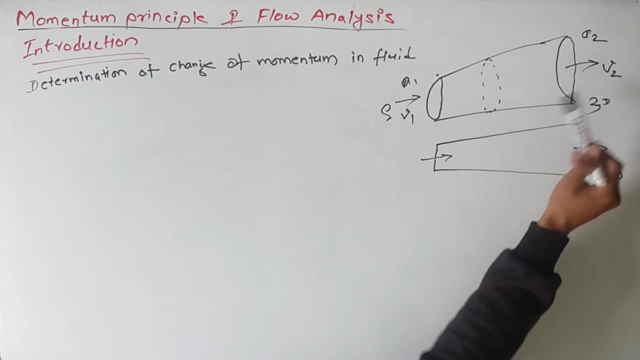 conditions such as your area change here is a1 here is a2 and build it here is u1 here is b2 these conditions are change but does not change with the time here we assume this area add inlet is a1 outlet is a2 so we can find here volume of liquid entering here in a small time 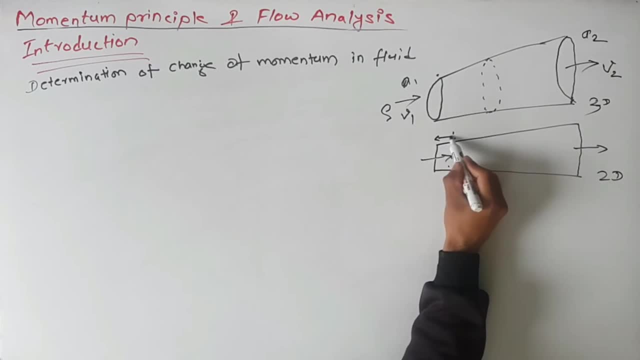 suppose here is the volume of liquid entering in a small section in a small time dt delta t 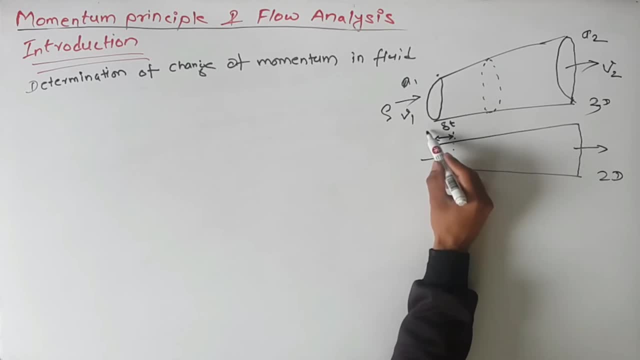 the which is equal to your velocity into time is the d distance travel into area similarly here b2 b2 delta t is the volume exit here so here i want to write 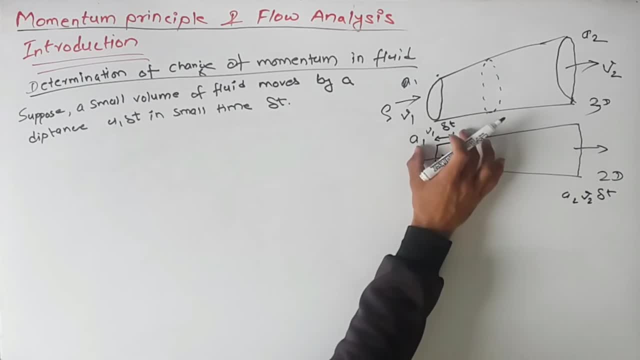 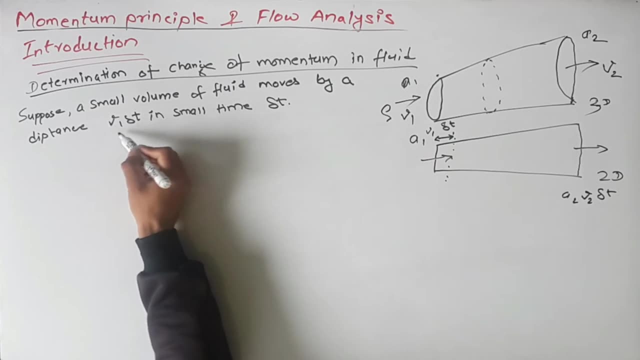 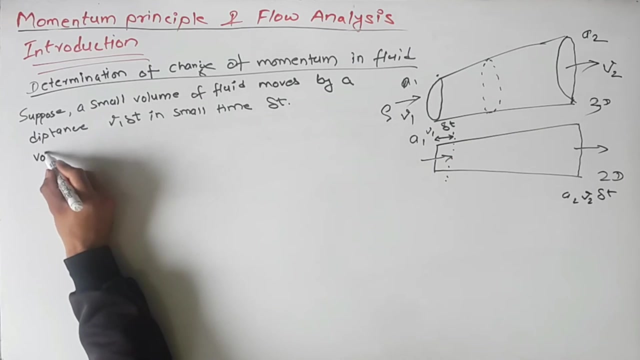 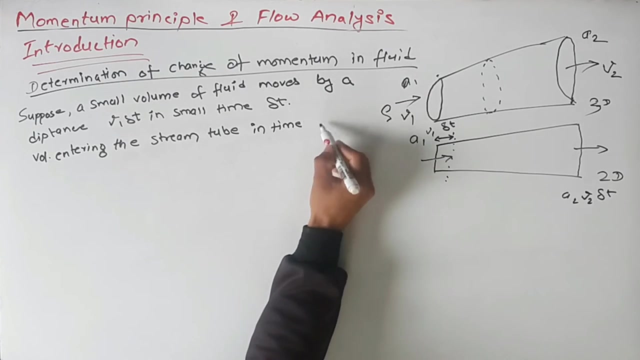 In small time delta t the distance u 1 here velocity is assume as v 1. So, here is v 1 v 1 delta t is moved by the fluid. So, we can calculate the volume here. Volume is equal to area at here a1 into the distance v 1 into delta t. This is the small distance is v 1 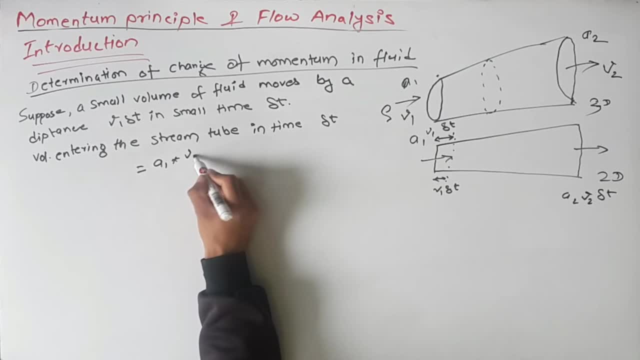 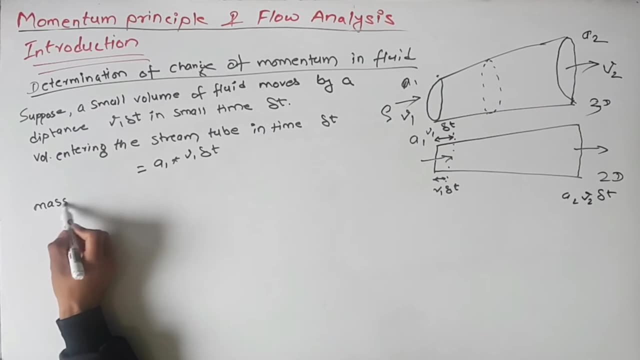 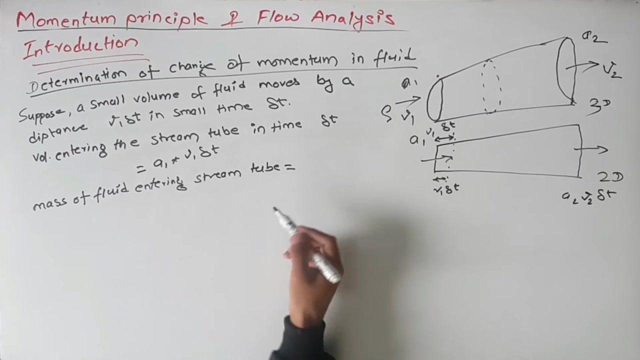 delta t volume is this. We have here volume. So, that we can find the mass entering here. Mass is delta t. So, we can find the mass entering here. So, we can find the mass entering here. Density into there is density is rho into volume. Volume is a1 u1 delta t. We have mass. 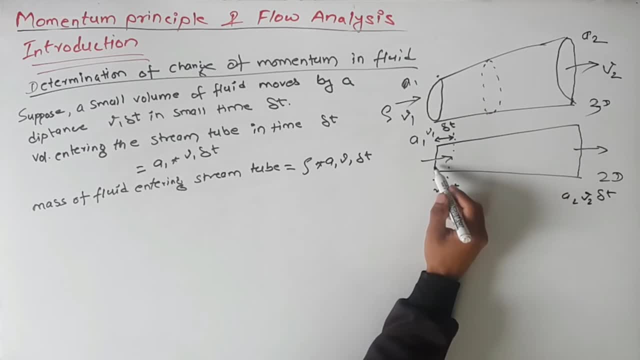 So, that we can find here momentum. Momentum of fluid entering the stream tube. 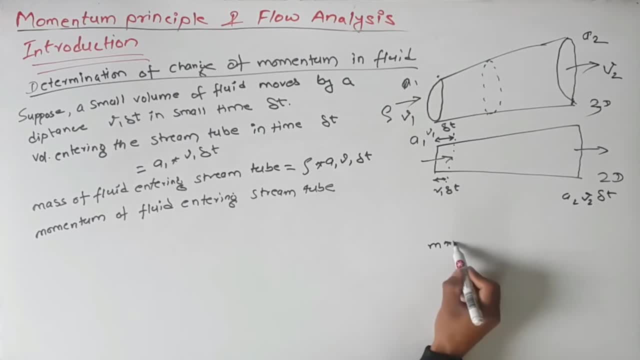 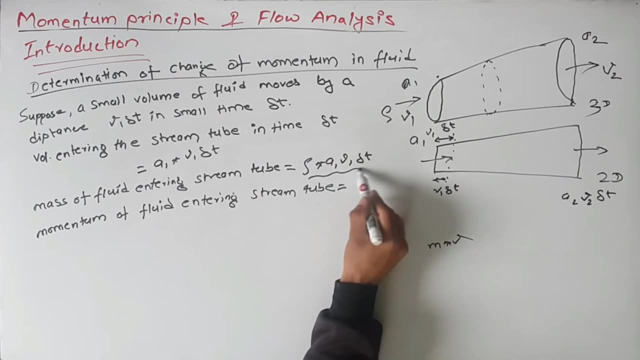 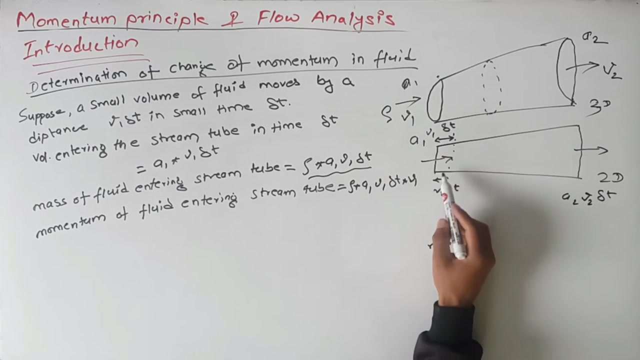 Momentum is product of mass and velocity. Density here is v 1. So, it is we have to multiply this with v 1. rho into a1 into v 1 into delta t into u 1. Here we found the momentum of fluid entering the. Similarly, we can find the momentum of fluid exiting this tube stream tube. 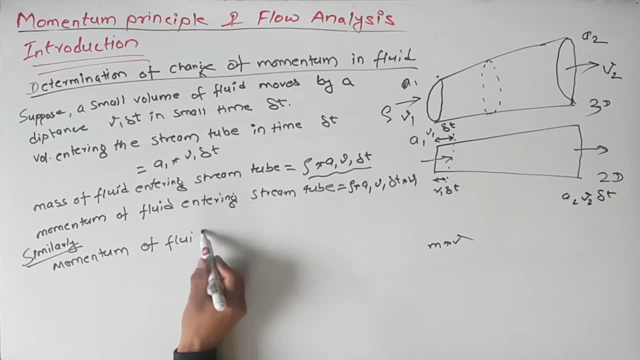 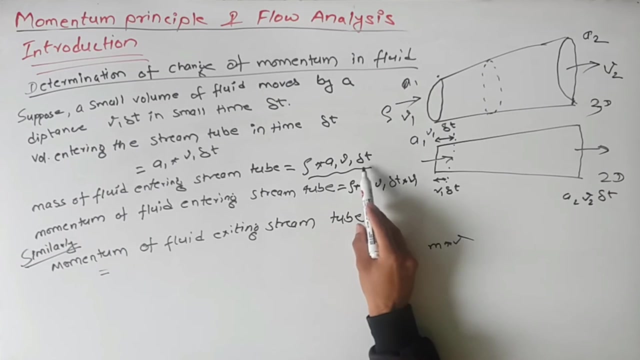 This is equal to here density into a2 into b2 into delta t into v2. This is equal to here density into a2 into b2 into delta t into v2. Similarly, we can do this procedure. 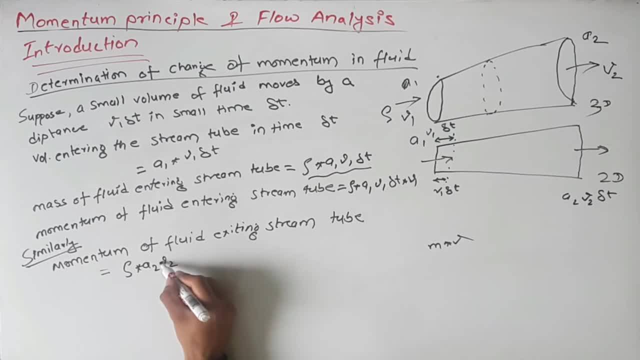 And here let me put the remaining Opening 90 degree circle. 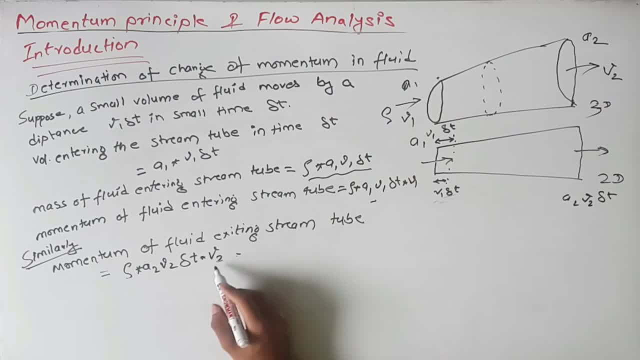 And here let meitz. Now, we canushx S 1, we can use Newton's second law. 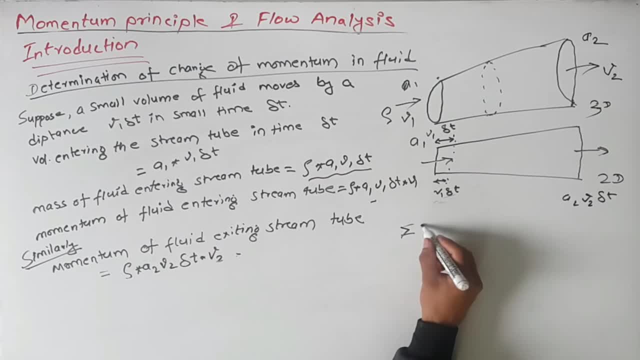 Newton's second law tells. So, sum of forces is equal to rate of change of momentum. 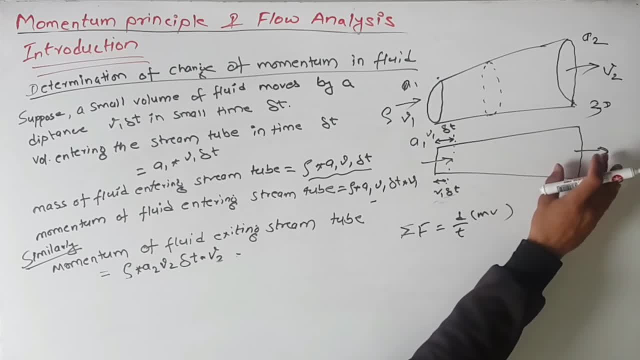 So, the distance from our intensive point to the room and ruptured point or the room on less than a distance from them is f mu phi Falcon Get x moment savior. So, here we haveithe ratio of pull current which is r. And this will be staying at this 3m, the length of this Sга. We quickly move zusada two or there is a small gap between them. They called these lengths to look and this state is our momentum. And part of the current momentum we have there as an interaction of momentum. 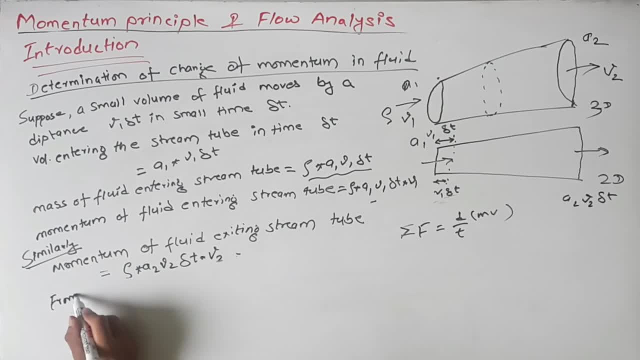 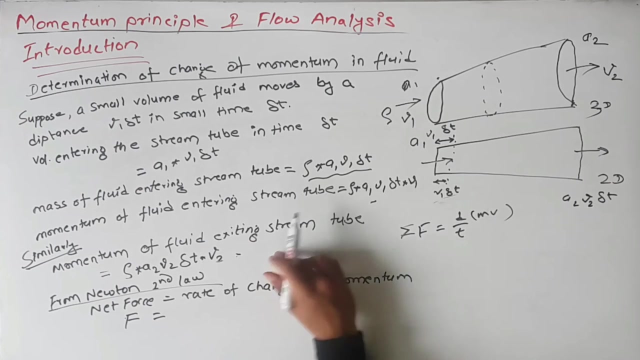 we use this Newton second layer. Net force is let F is the net force and rate of change of momentum, final momentum minus initial momentum upon small time delta t. 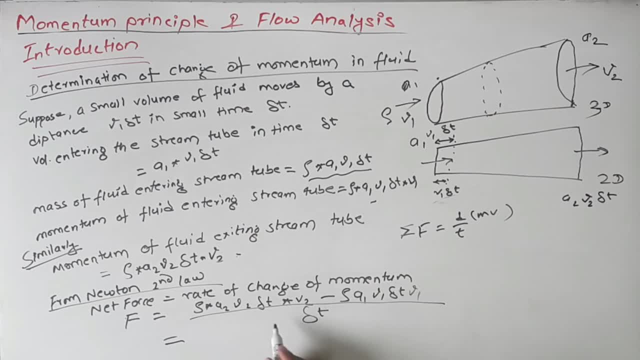 We have delta t small time. So that. Now we can use the continuity. Continuity equation. 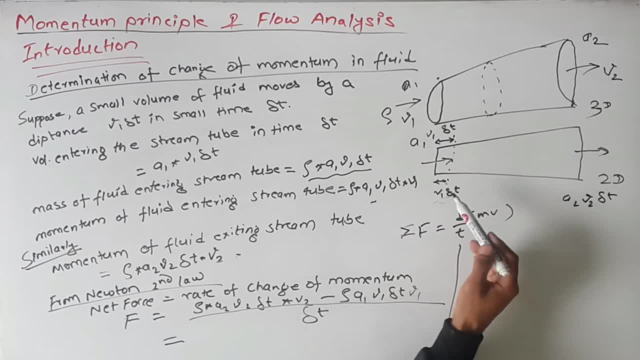 We assume this flow is non-uniform, steady and continuous. 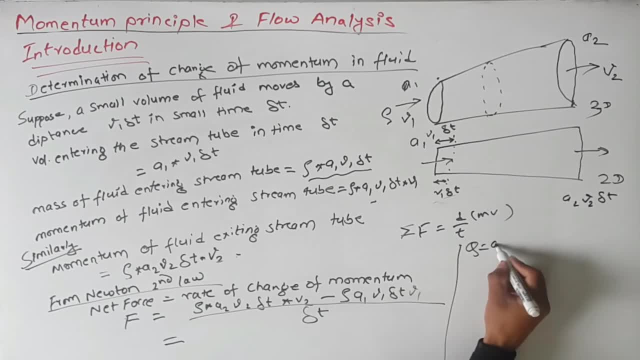 So by continuity equation we have Q equal to A1 B1 equal to A2 B2. 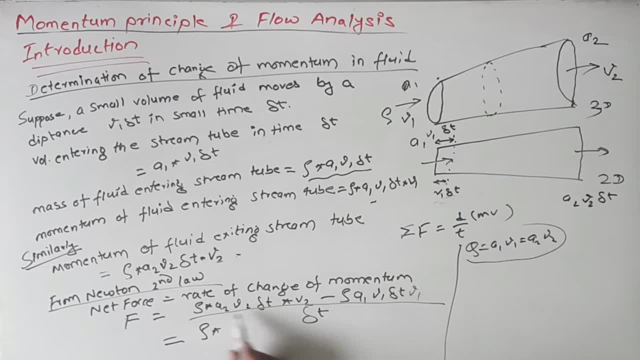 So we use this here rho into A2 B2 is Q delta t into B2 minus rho Q delta t B1 here upon delta t. This delta t, delta t upward we can take common and part with lower. So that no need to write here this delta t here. We have only remaining is rho Q B2 minus rho Q B1 is remain here. So rho Q is common here. So that. 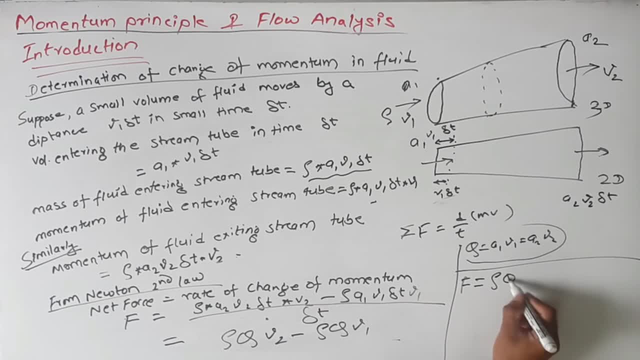 E of A is equal to rho Q B2 minus B1. In place of rho Q we can write m dot here. I want to show you how this rho Q is equal to m dot. 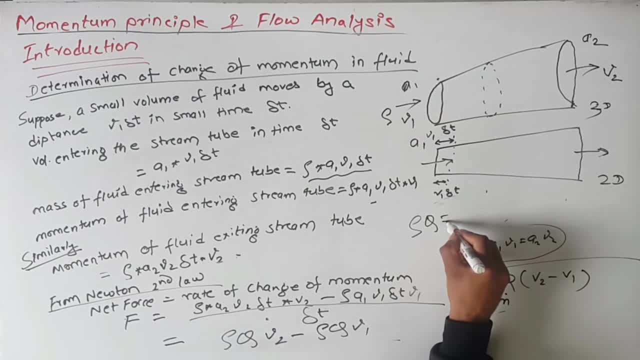 Rho density into B star. Rho Q equal to density. Density. Density. Density. Density. 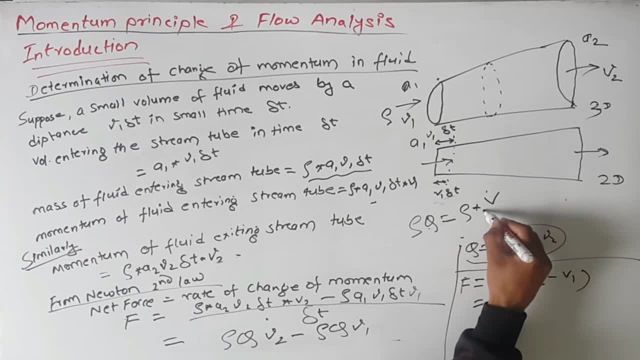 Rho is density into discharge is volume per unit time. And we have density into volume is mass and this upon time. 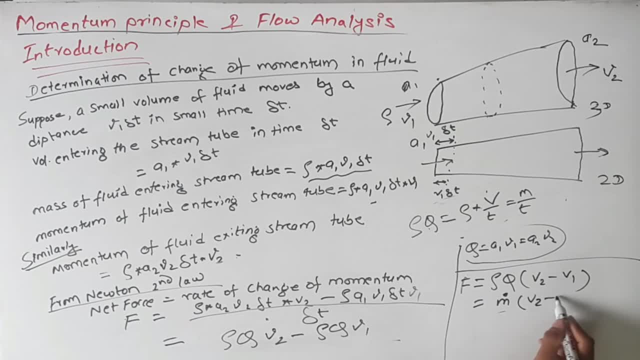 This mass per second is written as here m dot B2 minus B1. 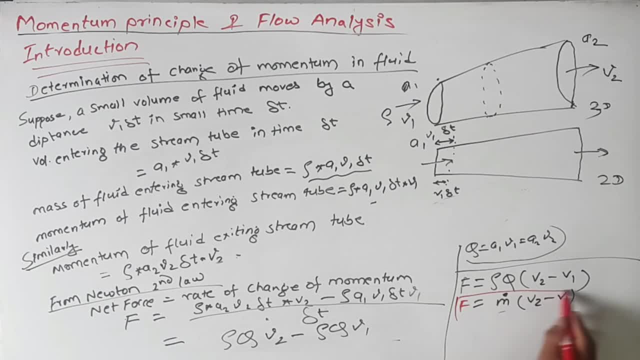 So we found here this force. Now we have this force. This is the force on the fluid. 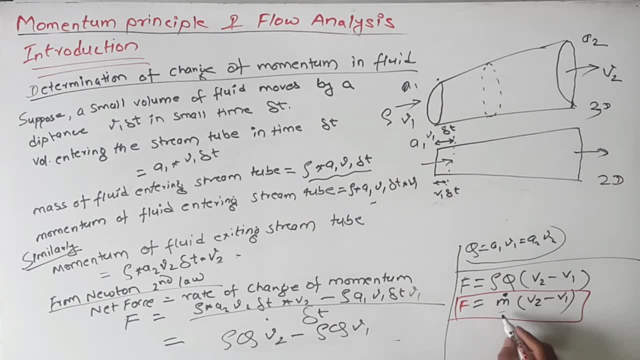 Here we analyze the mass per second entering and exiting. This is m dot. But in case of solid mechanics, we use whole mass of body. 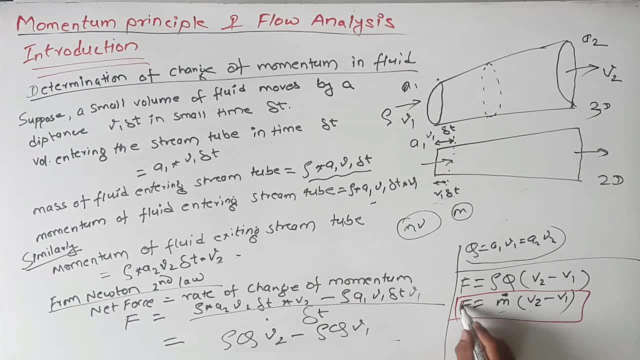 This is equation of force exerted by the fluid in two dimensional. 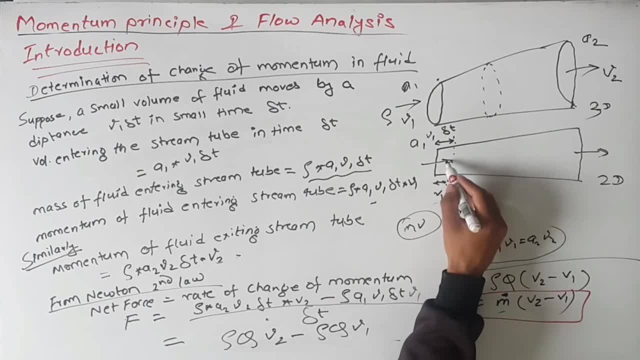 Sorry, in one dimensional. Here velocity into mass. This is mass. This is mass. Initial velocity and final velocity are in same direction. So it is one dimensional flow. 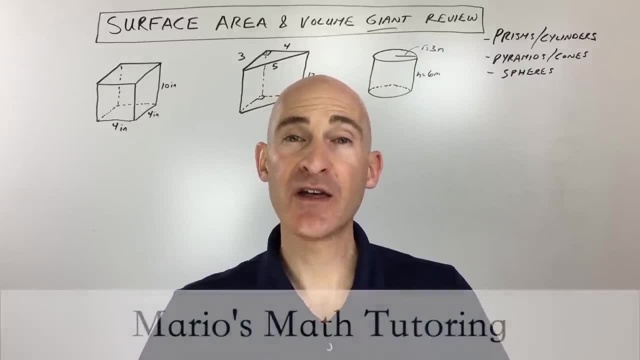 In this video, you're going to learn how to find the surface area and the volume of three-dimensional figures. We're going to talk about cones, we're going to talk about pyramids, we're going to talk about prisms and cylinders and spheres. So let's get into this video and 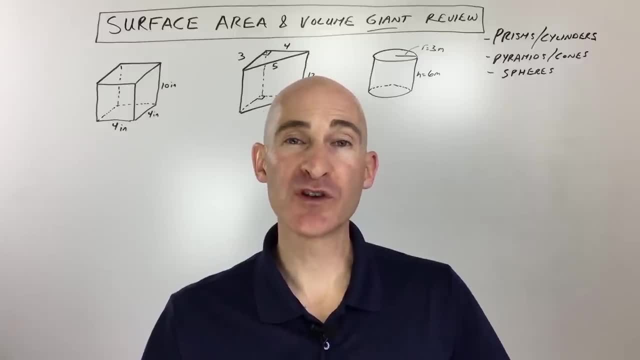 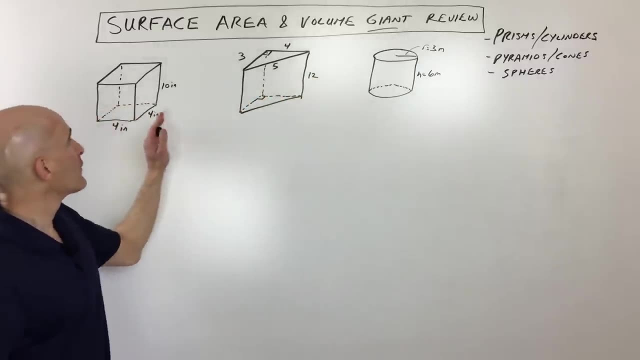 we're going to go through the formulas. I'm going to show you an easy way to remember these formulas and how to group them together so that you don't forget them and you'll be able to solve these problems easily. So let's get into the first group of problems, The first group we're talking about. 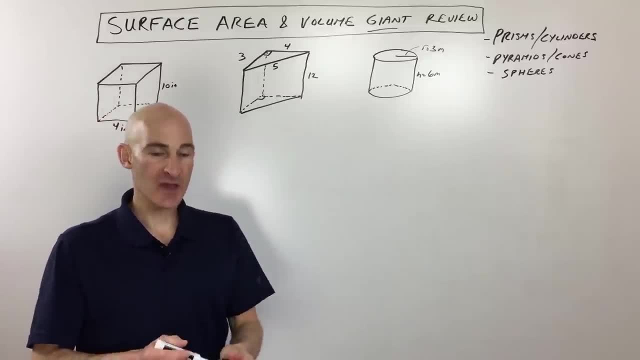 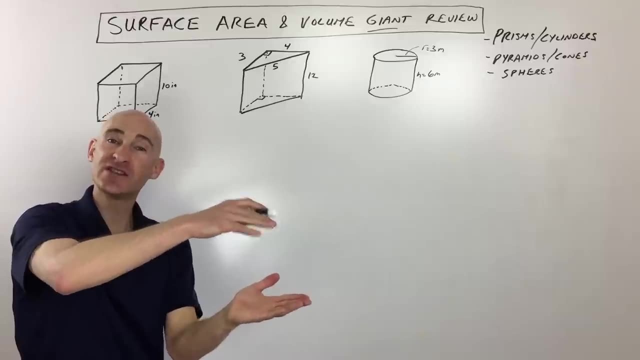 prisms And basically what a prism is. a prism is a figure, a three-dimensional figure, where the two bases are parallel and they're congruent. So that means they're the same size and shape and they're parallel. they don't cross if they were to continue to go, and they're separated by